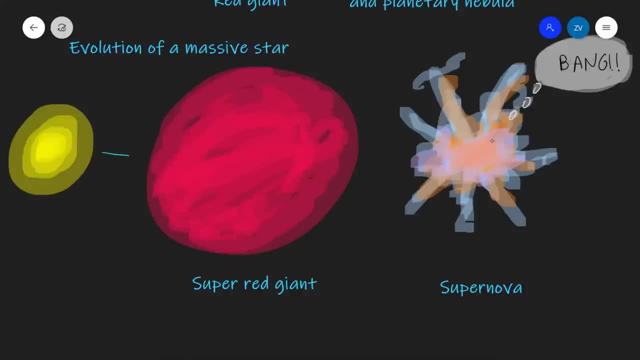 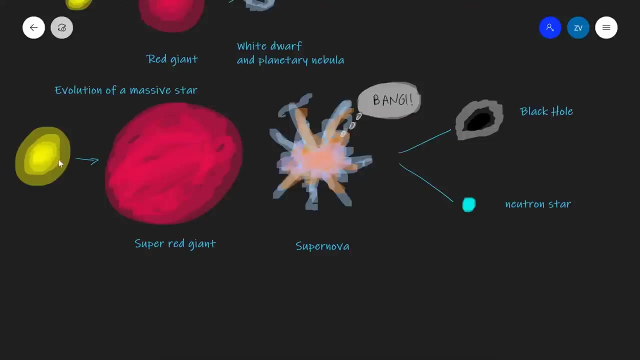 turn into a super red giant, which is shown here. When the super red giant doesn't have any more fuel left, it ends up in a gigantic supernova explosion. Depending on the initial mass of the star, the final outcome will either be a neutron star, if the original star is a little 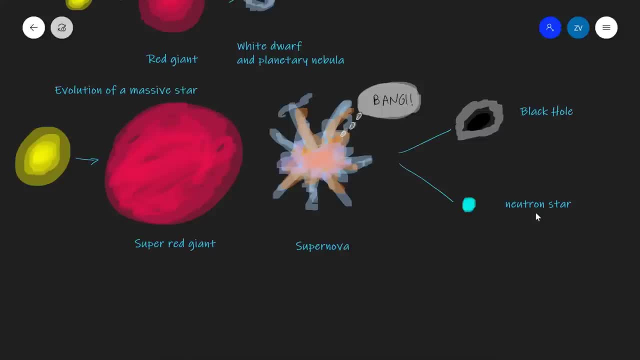 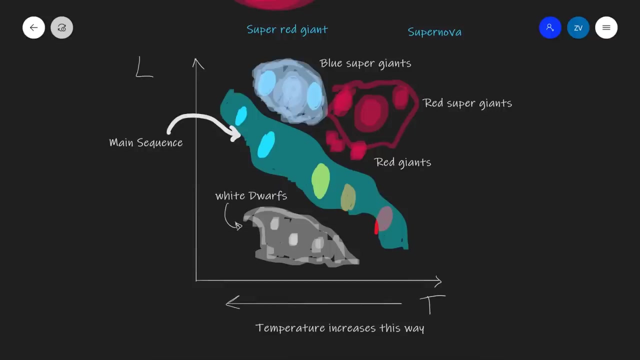 bit lighter, or a black hole if the star is heavier still. Both of these objects are very, very dense, and a black hole will actually have infinite density. The way of categorizing all of the stars is provided by the Hertzsprung-Russell diagram, which is presented over here. On the y-axis we 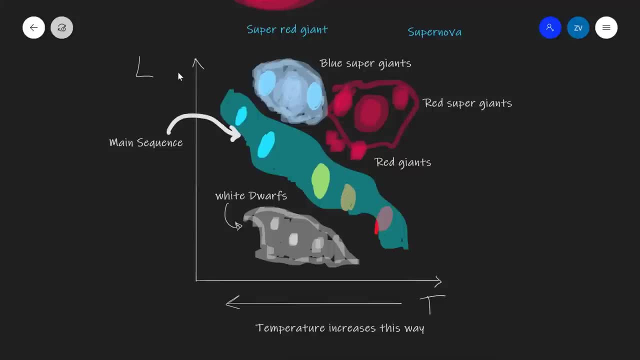 have luminosity, which is the total power radiated by the star On the x-axis. we have temperature. In a Hertzsprung-Russell diagram, the temperature increases to the left, so this is really important. For instance, blue supergiants are further on the left compared to red supergiants. 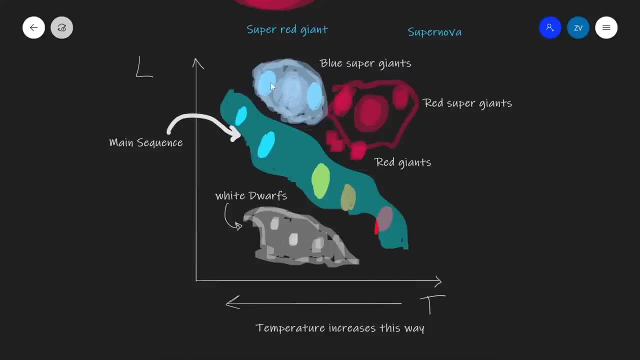 therefore, blue supergiants have the higher temperature. Additionally, we need to be able to remember and identify the different features of this graph. The main diagonal is the main sequence. This is where the star will spend the vast majority of its life cycle When it runs out. 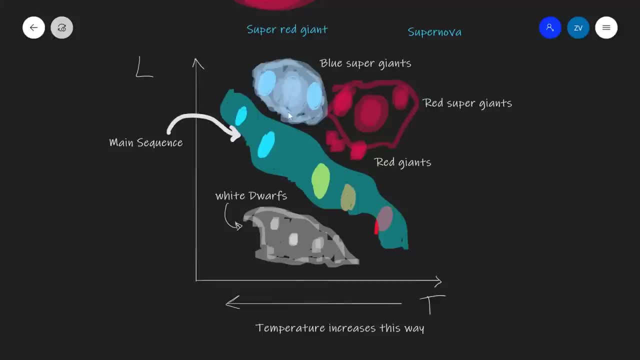 of fuel. it will run out of fuel. When it runs out of fuel, it will run out of fuel. When it runs out of fuel, it will either turn into a red supergiant or a blue supergiant and eventually, depending 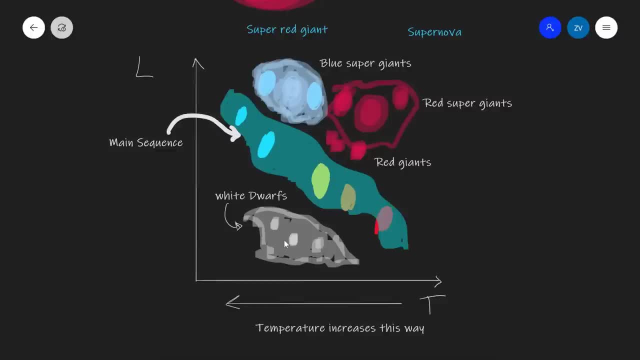 whether that's possible. it may turn into a white dwarf. White dwarfs are presented by this lower left-hand region of the Hertzsprung-Russell diagram. Now, what actually determines whether a star is going to turn into a white dwarf? Well, it's going to depend on whether the star is going to turn into a 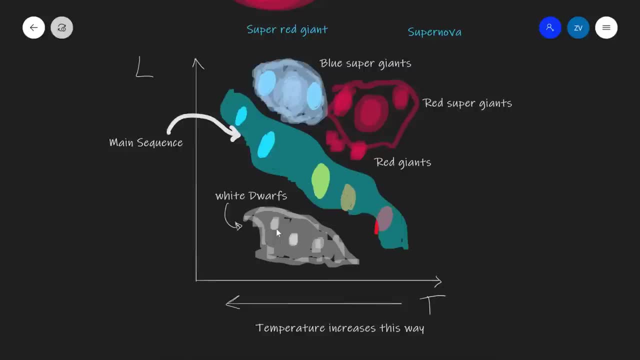 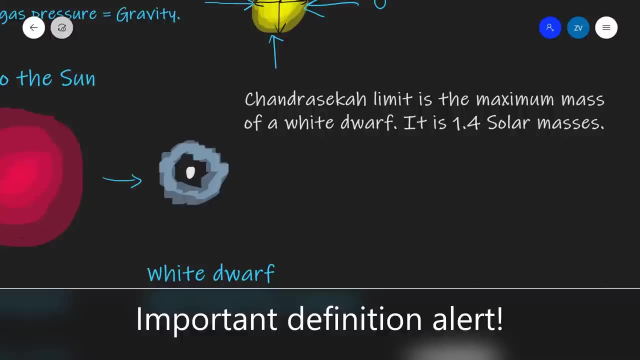 white dwarf or not. Let's revise the Chandrasekhar limit. This here is a really important definition. The Chandrasekhar limit is the maximum mass of a white dwarf star, and that is 1.4 solar masses. If the Chandrasekhar limit is exceeded, we'll get different objects, for instance, 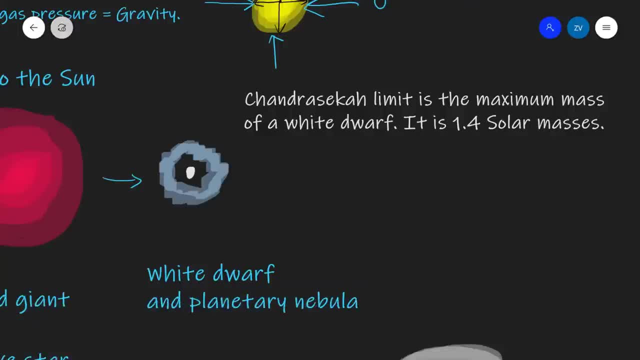 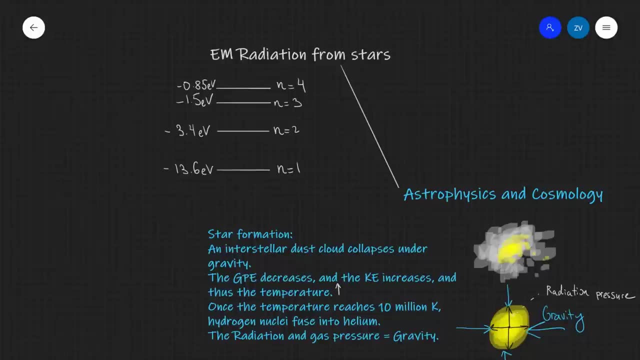 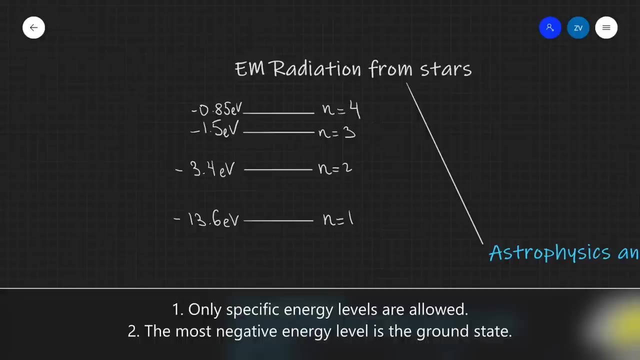 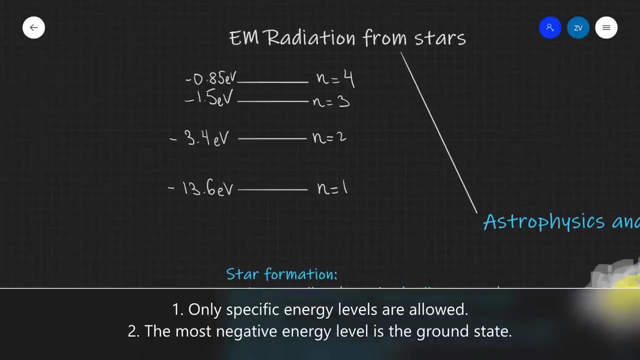 a neutron star. Now that we have finished with stars, what I would like to revise next is EM radiation from stars. The first aspect that we need to revise is the fact that electrons can occupy different energy levels within the atom, and only certain energy levels are allowed. So 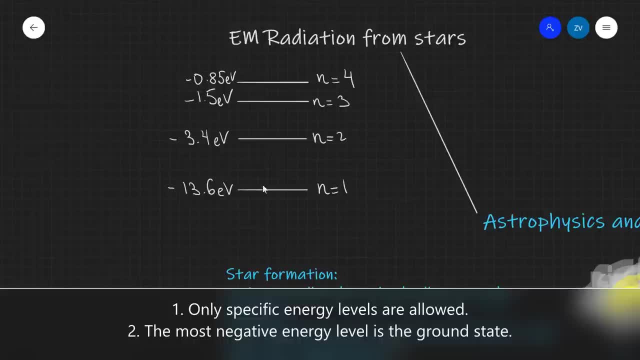 in the case of hydrogen, for instance, these are the first energy levels and the electron can only occupy those specific energies and none of the energies in between. The most negative state is known as the ground state, like so. So this is the ground state, and if we keep, 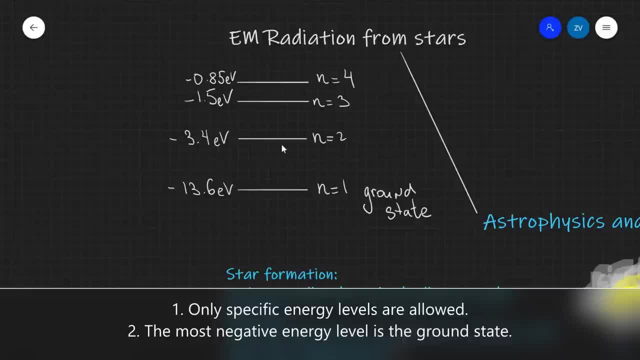 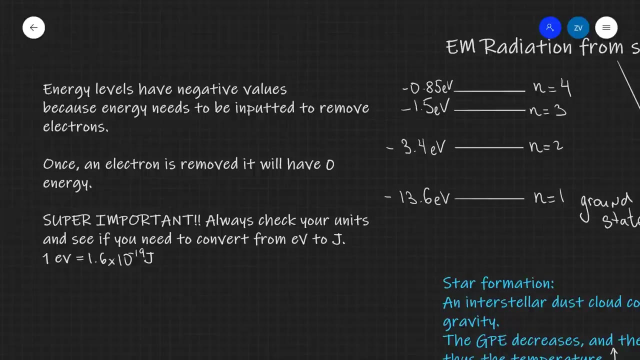 inputting energy into an electron, it will go up in energy levels until eventually it reaches zero and the electron is ionized, In other words, it escapes the atom. It's also really important to say that energy levels have negative values because energy needs to be inputted into the atom. 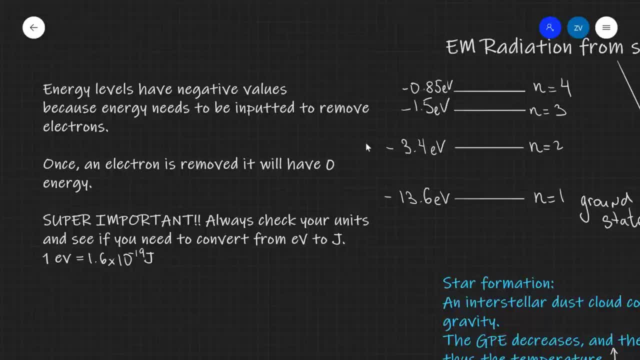 and the electron needs to be put into the system to remove electrons. As I said, once an electron is removed, it will have zero energy, So, which is super important, please always check your units and see whether you need to convert from eV to joules, For instance, if you want to calculate. 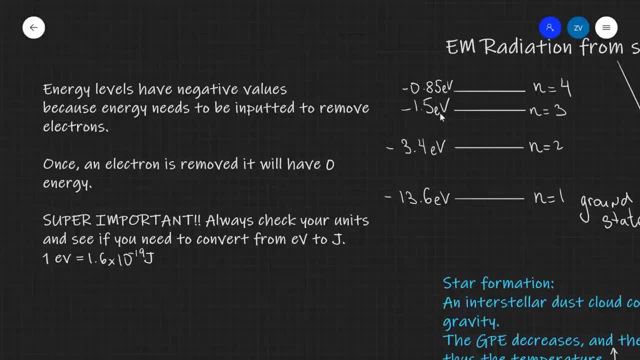 anything from this graph later on. in order to get an answer into SI units, you will need to convert from electron volts to joules. The conversion factor is multiplying by 1.3, which is 6, times 10, to the power of minus 19,, which is the electron charge. Because of conservation of 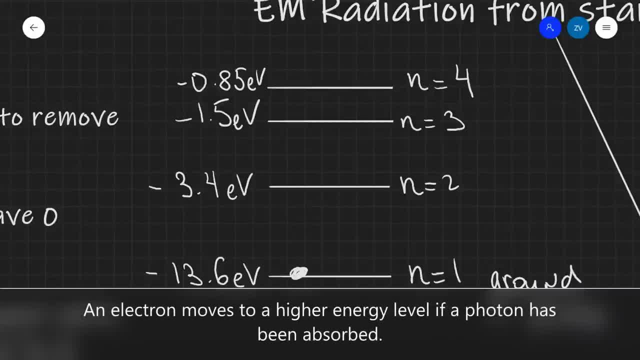 energy. if an electron jumps up an energy level, for instance, if it went from energy level 1,- the ground state- to energy level 2,- right over here- this means that a photon must have been absorbed. On the other hand, if a photon 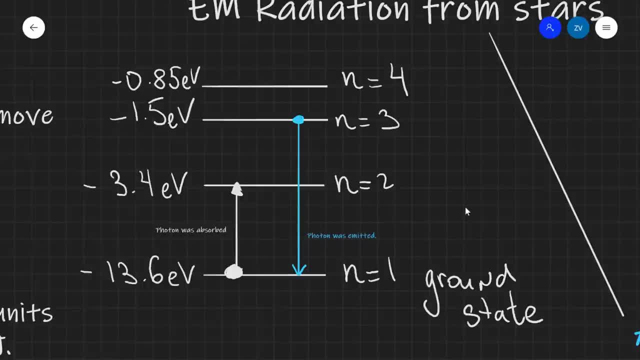 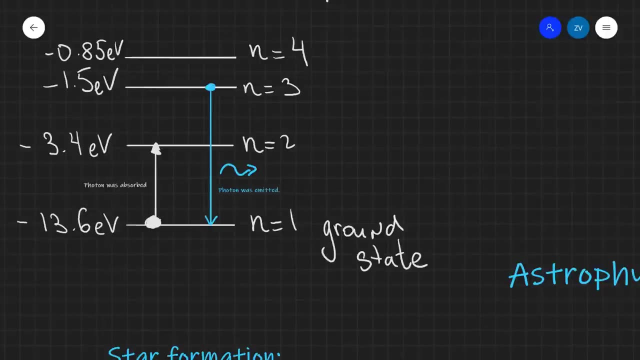 On the other hand, if an electron goes down in energy level, for instance, from n is equal to 3, to the ground state, this means that a photon must have been emitted due to energy conservation. Let's focus on the first transition in which the photon was absorbed. Let's call this one. 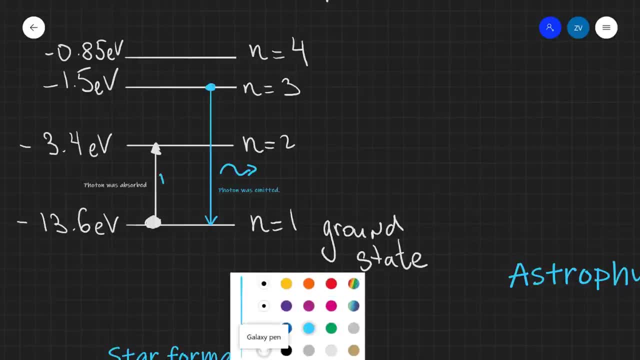 transition 1, for instance, and just over here we are going to do some calculations. So for transition 1, the difference in energy from minus 13.6 to 3.4 electron volts is equal to 10.2. 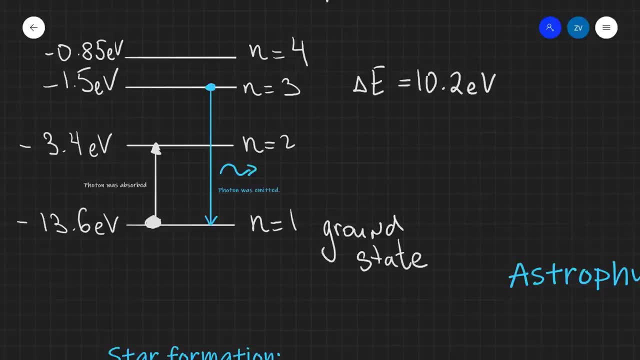 EV. We could use that to calculate the frequency of the photon that was absorbed. simply by setting this energy delta E equal to the energy of a photon which is equal to HF, We could just rearrange the energy for the frequency and then we could just go back over to transition 1, and we could. 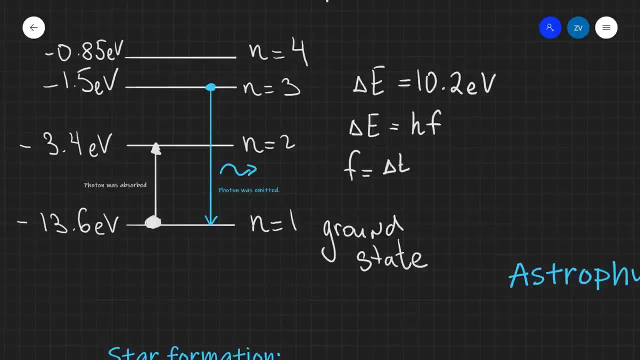 and we can get that. the frequency is equal to the change of energy divided by Planck's constant. It would be very, very important to convert the energy from eV to joules, So this will be equal to 10.2 electron volts. so converting to joules we'll need to multiply this. 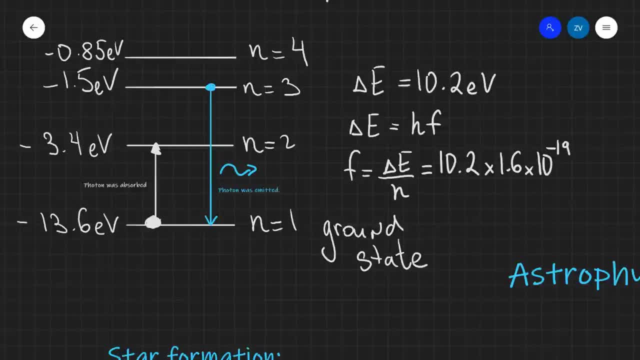 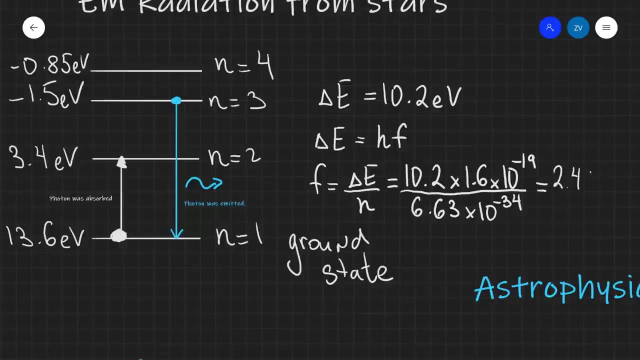 by the elementary charge, like so. and then we're going to divide by Planck's constant, which is 6.63 times 10 to the power of minus 34,, giving us 2.46 times 10 to the power of 15 hertz. 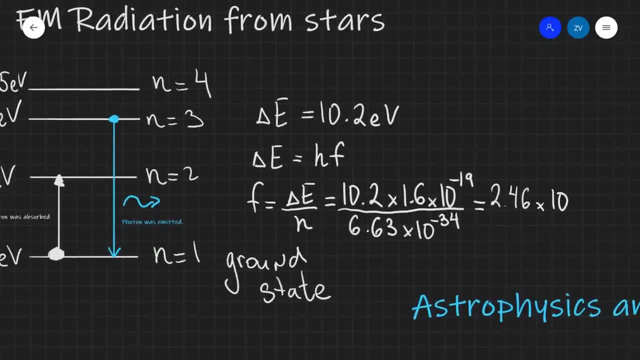 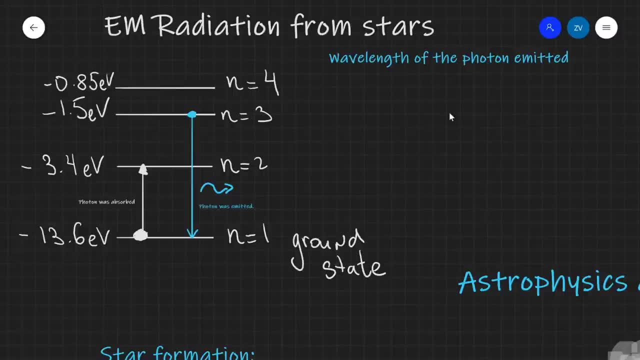 So let's write this down over here: 2.46 times 10 to the power of 15 hertz. We could also focus on this second transition, the one here in blue, in which a photon was emitted, For instance. we could try and calculate the. 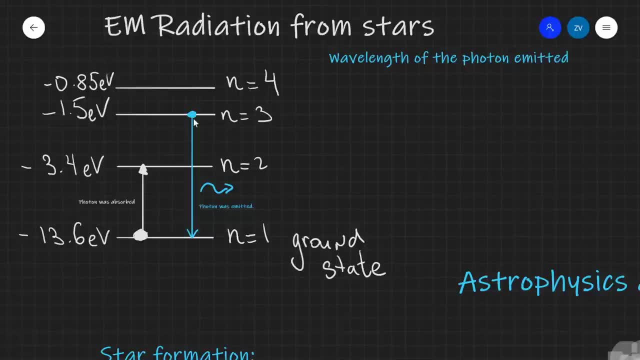 wavelength of the current, The wavelength, this time, of the emitted photon. The way we're going to do this. first off, we need to find our difference in energy. So 30.6, take away one and a half is going to give us 12.1.. 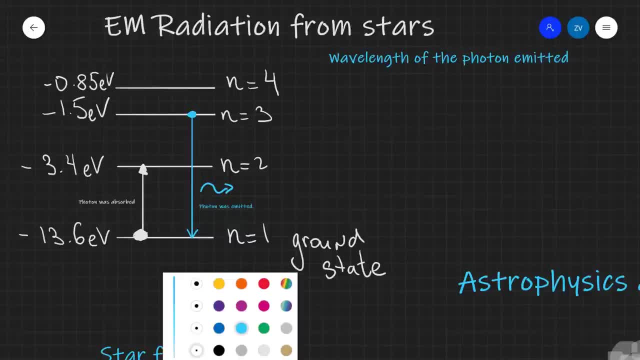 That's a little bit too big. let's try again. It's going to give us 12.1 eV. Now we can set this change of energy equal to hc over lambda, And all we need to do really is just rearrange for the wavelength. 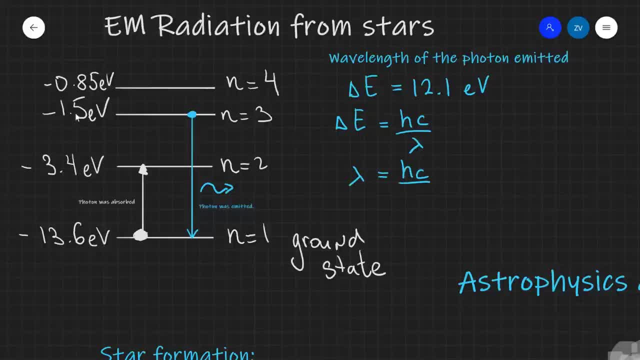 The wavelength will be equal to hc divided by the difference in energy, giving us h, which is 6.63 times 10, to the power of minus 34 times the speed of light, which is 3.0 times 10 to the power of 8.. 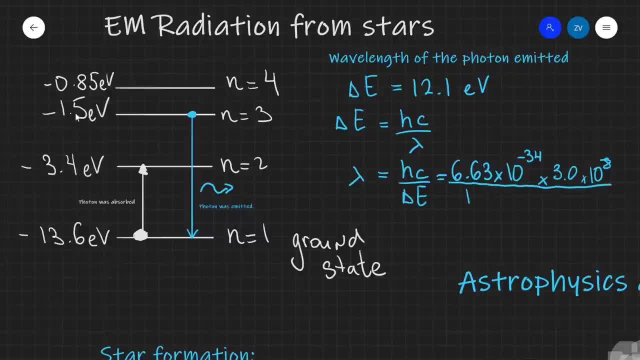 Divide that by delta e, which is 12.1.. Remember, we need to convert this to delta e, which is 12.1.. So we convert that to joules, So multiplying by the elementary charge, which is 1.6 times 10, to the power of minus 19.. 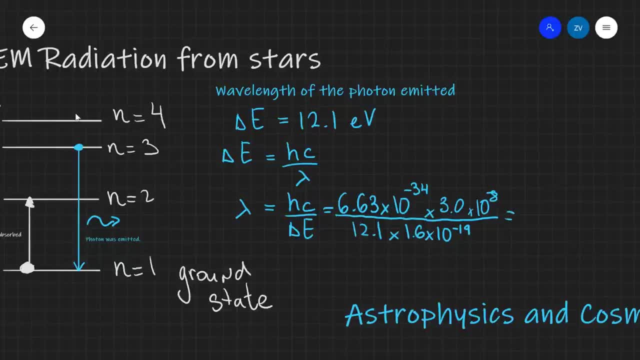 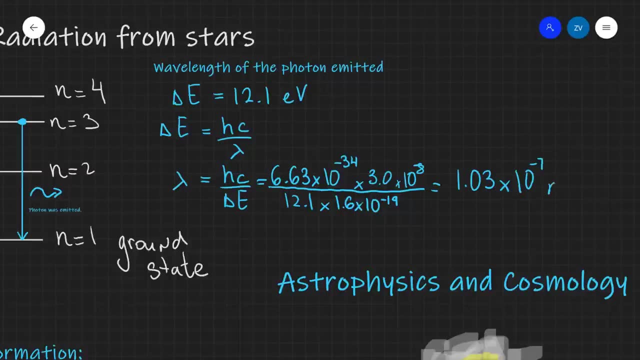 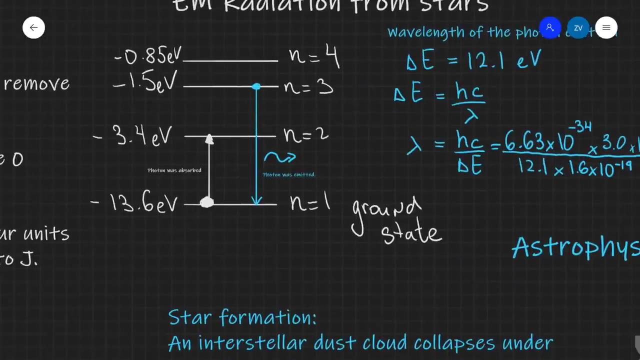 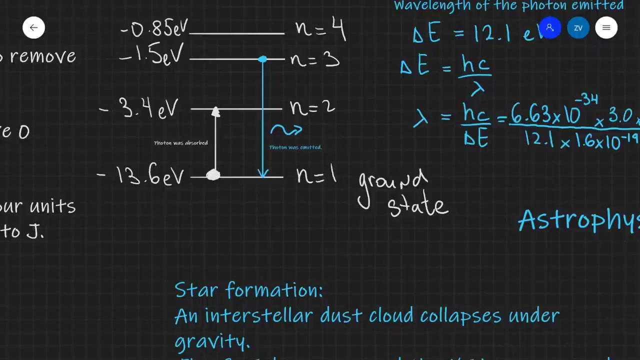 And if we put that into a scientific calculator, giving us 1.03 multiplied by 10 to the power of minus 7 meters. In general, with those problems, we always set the change of energy equal to the energy of a photon, leading us to those two equations which we've just used. 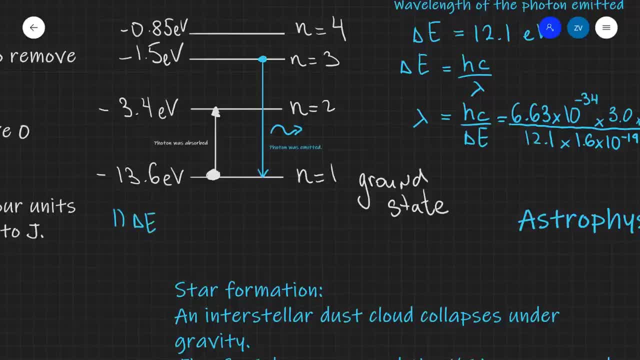 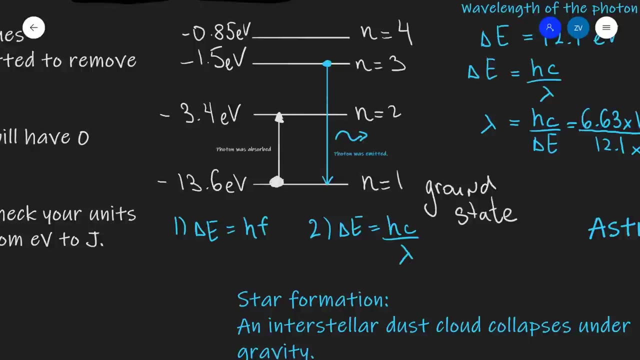 The first one is that delta e is equal to hf. If we're looking for the wavelength, or if we're given the wavelength and we need to calculate something else, delta e is equal to hc divided by lambda, Talking about the energy levels and the transitions between them. 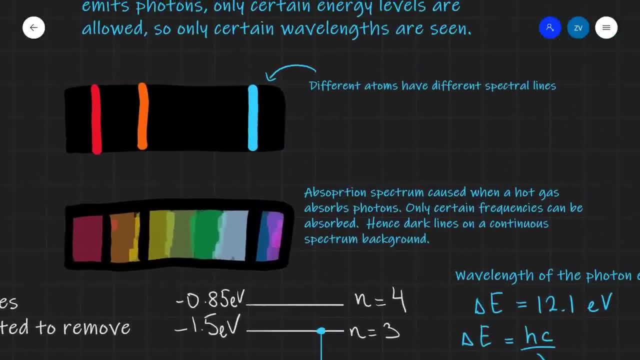 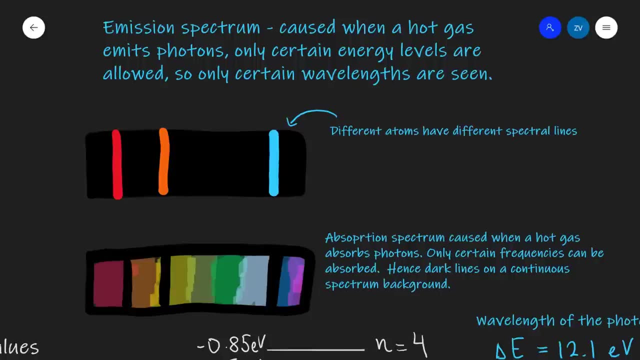 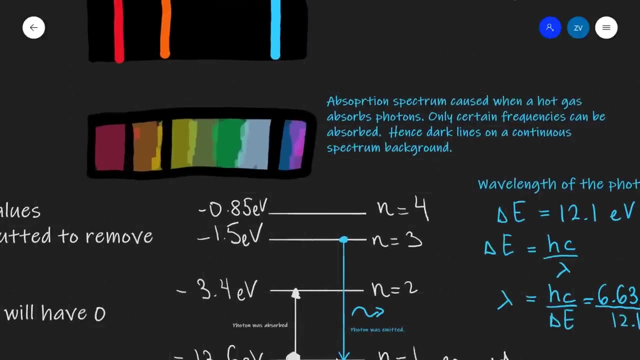 we need to mention the continuous and absorption spectrums. First off, let's start with the emission spectrum. This is caused when a hot gas emits photons. Because only certain energy levels are allowed, such as in this diagram, You can only go, let's say, from here to here, from here to here, from there to there. 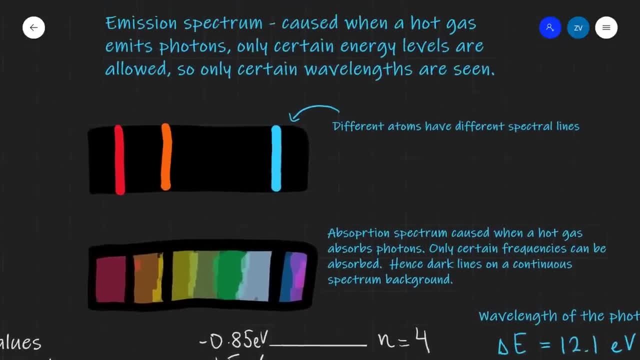 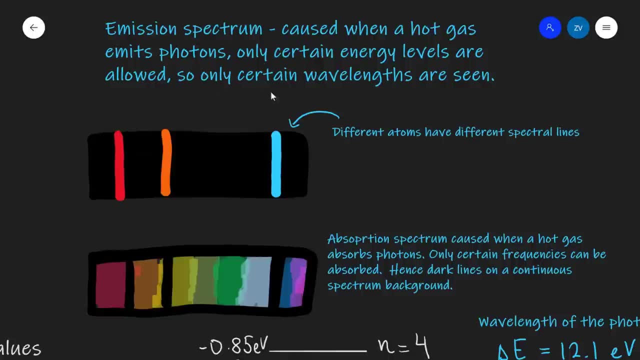 Only certain wavelengths can also be emitted. So therefore, if we heat up a hot gas, we're only going to see certain wavelengths, For instance this one, this one and this one, and no other ones. Therefore, the emission spectrum spectrum looks the way it does, with coloured vertical lines on a dark black background. 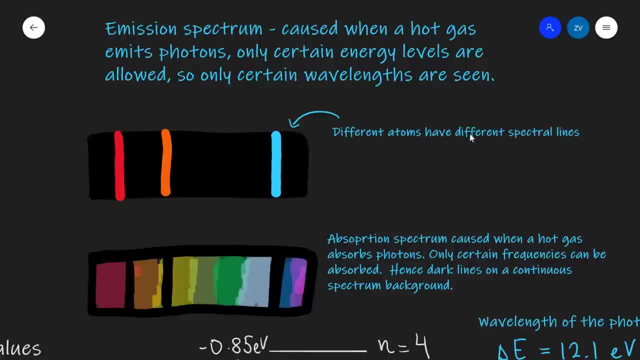 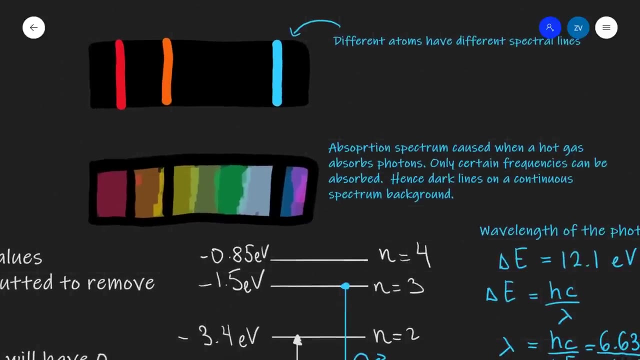 Different atoms can have different spectral lines and we can use those to identify them. So, for instance, helium's spectrum is going to look different from hydrogen's etc. and we'll be able to identify them. We can also have an absorption spectrum, which is caused 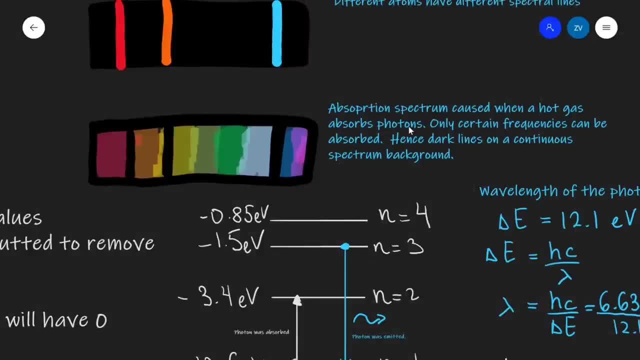 when a hot gas absorbs photons, For instance in the solar corona, the solar atmosphere will be able to absorb some of the photons that are being emitted from near the core of the Sun. Because only certain frequencies or wavelengths can be absorbed, then they 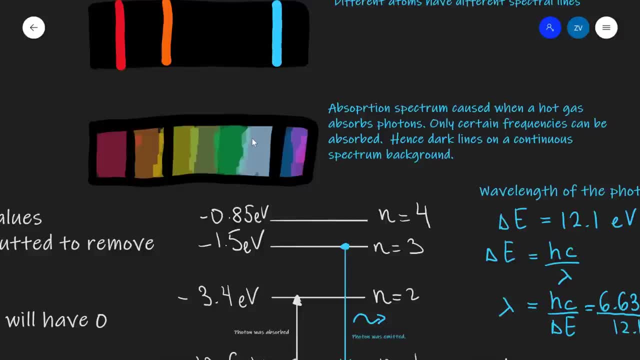 will correspond to those dark lines. Therefore the absorption spectrum looks like such. It is dark black lines on a continuous spectrum background. Colloquially, continuous spectrum will compose of all the different wavelengths, so it looks similar in the visible range as: 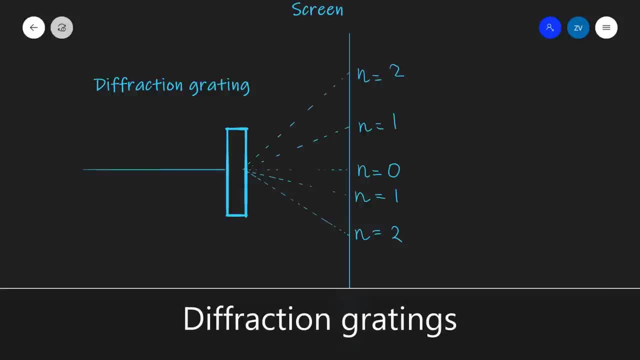 a rainbow. One way to find the wavelength of an incoming light in order to analyse it is via a diffraction grating. Remember, diffraction is the spreading of light as it passes through a gap or around an obstacle. A diffraction grating is going to have multiple different slits along all around its surface. 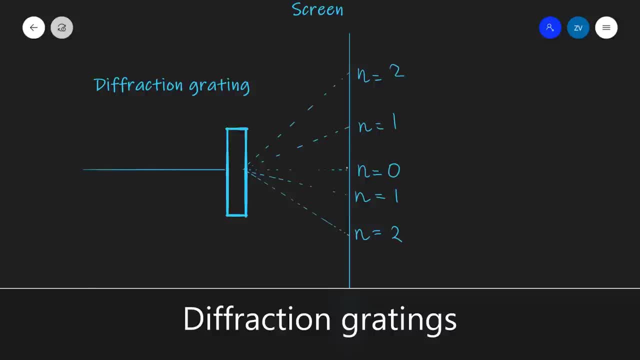 and once the light passes through, it is going to spread, resulting in a diffraction pattern which will be seen on the screen. The equation which governs this is that d sine of the angle theta is equal to n times lambda. Let's analyse this equation. 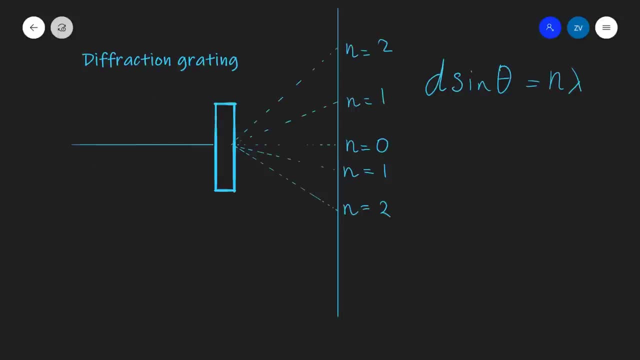 D in this equation is equal to n times lambda. Let's analyse this equation. D in this equation is equal to 1 over the number of lines per metre. This is really, really important. Let's say that this diffraction grating had 300 lines per millimetre. This would mean: 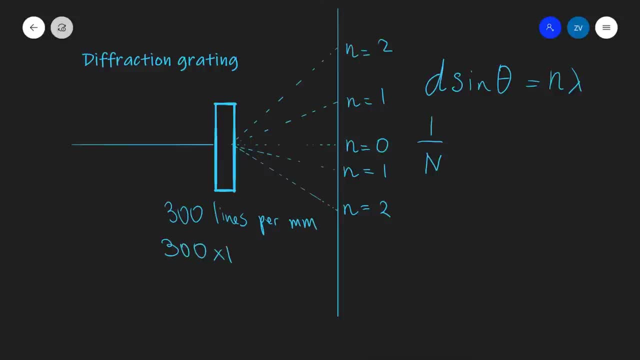 that it will have 300 times 10 to the 3 lines per metre. In other words, d really is equal the spacing between the individual lines. so 1 over n is in this case going to be 1 over 300 times the power of 3. theta is the angle that corresponds to the order. 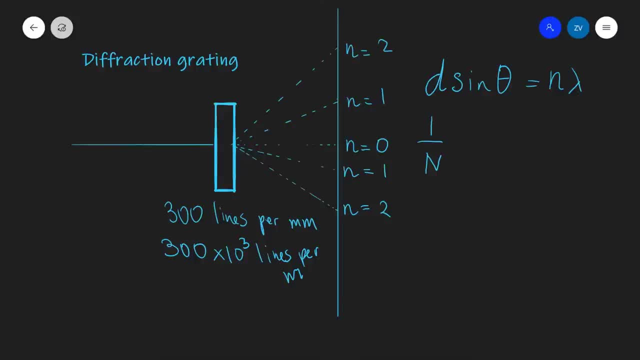 of the diffraction, for instance, for interested in the position of this particular fringe, our theta is going to be this one over here. let's give it a number. let's say that this one here is 25 degrees. we want to use that in an equation in in a minute. so this is the angle theta and, as I said, is the order. 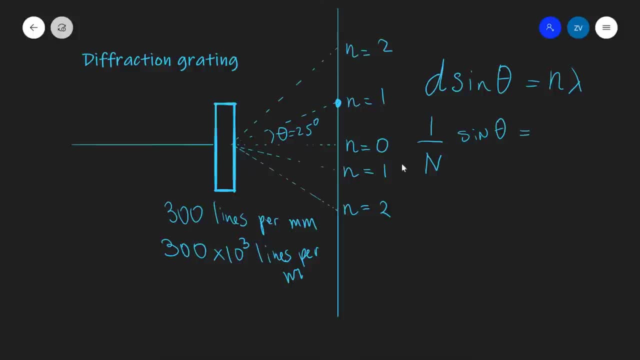 of diffraction doesn't really matter whether we choose this side or this side, because this angle here will be the same as the other angle and lambda is the force of the angular magnitude. then the angle of the angle, theta, is equal to the, the wavelength. we could use that to find the wavelength of the particular light. 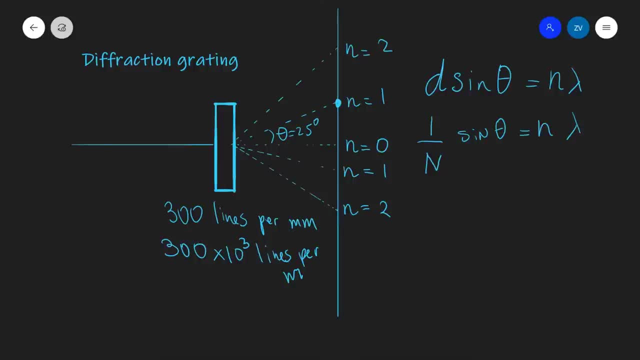 so let's do that for the values given for the first order of diffraction. so 1 over n will be equal to 1 over 300 times 10 to the power of 3, like so, multiplied by the sine of 25 degrees that's going to equal to the first order. so n is 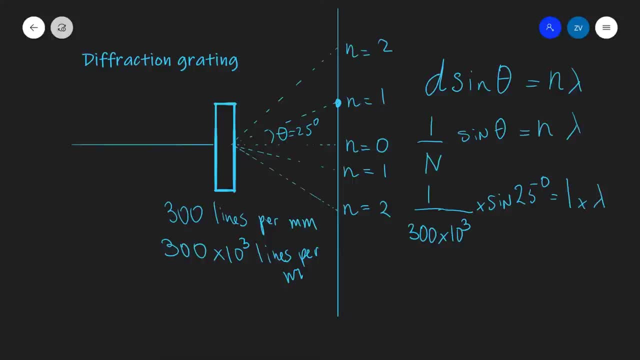 equal to 1 times the wavelength. all we need to do really is just put that into a calculator and I'll be able to find the wavelength of that particular light. so lambda will be 1 over 300 times 10, to the power of 3 times the sine of 25. 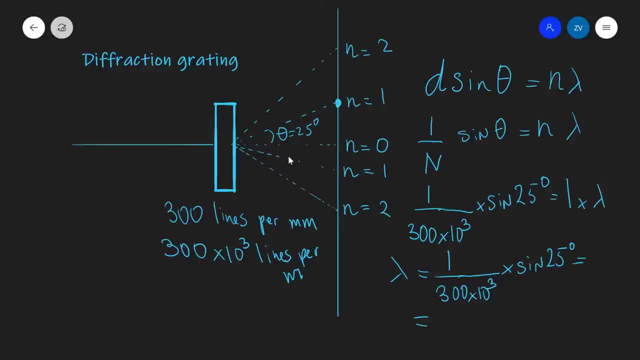 degrees and if we put that into the calculator we'll be able to find the wavelength of the particular light. so if we put that into a calculator we are going to get 1.4 multiplied by 10 to the power of minus 6 meters. we could use a. 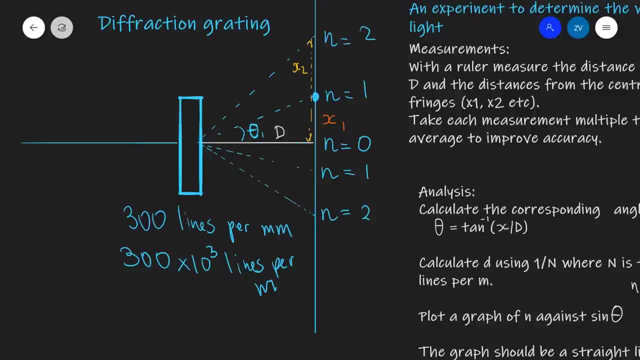 diffraction grading for an experiment to determine the wavelength of the light that has gone through the diffraction grading in practice as well. this could be used to determine what wavelengths are within the light that is incoming in telescopes from stars. let's have a look at this. 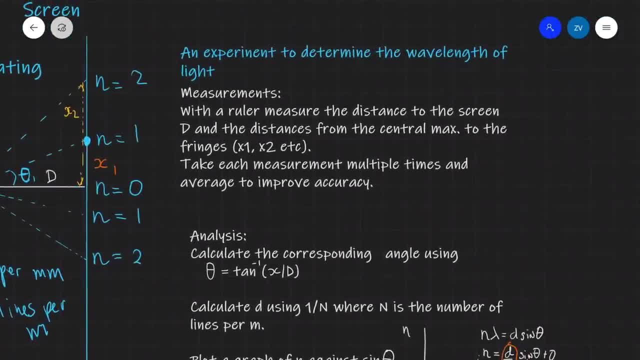 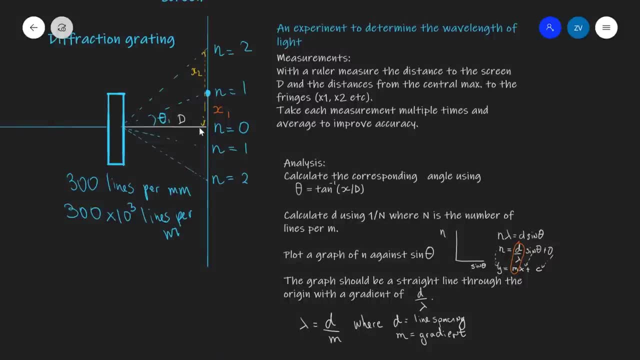 let's have a look at this experiment. so we're going to need to take certain measurements with a ruler. we're going to measure the distance to the screen D and then the distance, the distances from the central maximum to the individual fringes in practice. this is good. this is going to be X 1 for this distance over here, and it's going to be. 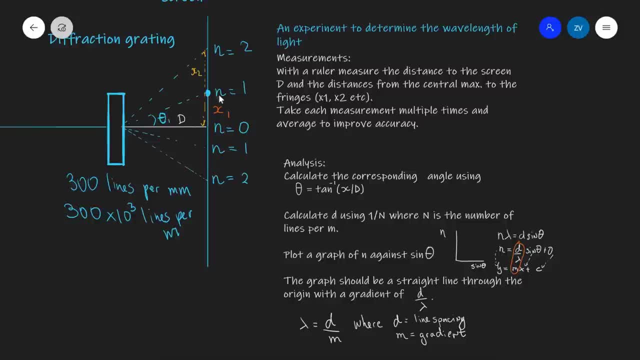 X 2 from the distance from the point n is equal to 2 to the central maximum. as always, we're going to take multiple measurements and we're going to average them each time to improve the accuracy in terms of the analysis. we can calculate the corresponding angle using: 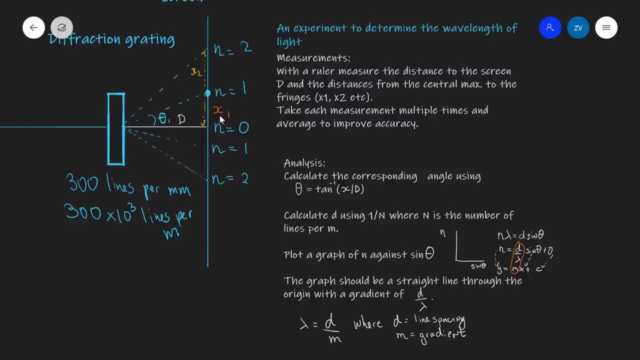 the fact that theta is going to be the inverse tan of X divided by D, where the distance X will correspond to the distance of the individual fringe to the central maximum. why is that so and just explain maybe a little bit about that in the next video. 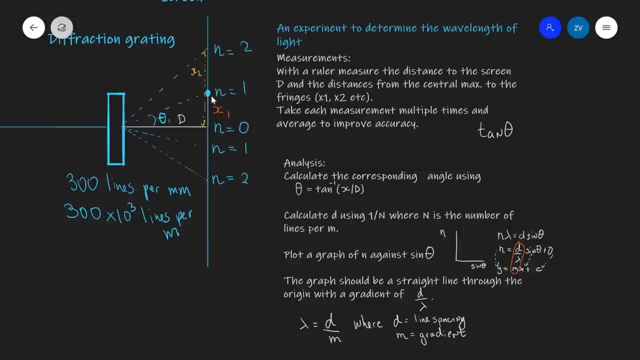 so that means that the angle in which this ح here takes place will be was, which is literally the angle in which this berth. Now, if we calculate the angle in which we have the straight line gathered using that inverse function, it will beela 00XIn closer with. 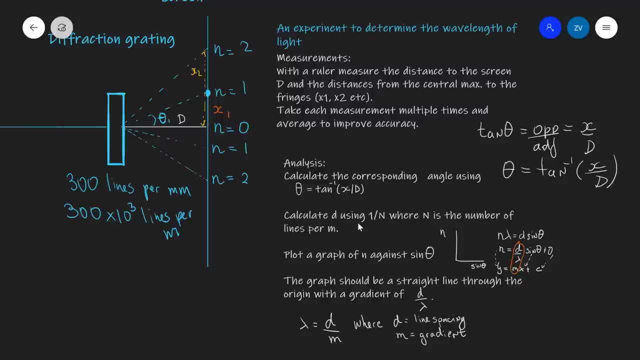 the Red, crossed over here Z, or the orange one which is available at this level of this chat engine. Let's see if Normally we can get the number of lines per millimetre from the actual diffraction grading. It will normally set on the diffraction grading itself. 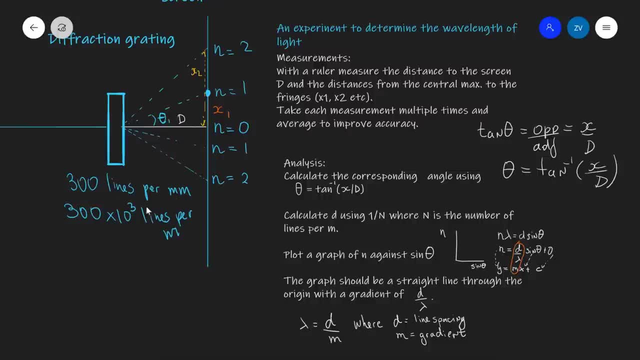 And that will be 300 lines per millimetre in this case, for instance, or 300 times 10 to the power of 3 lines per metre. And this over here is our n, so n is equal to that. So once we have our angles- so let's say we've calculated- we have essentially a table of x, d and the angle theta. 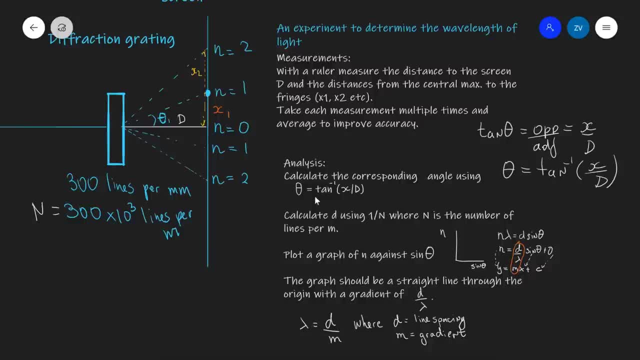 Let's say we've calculated 3 or 4, or hopefully as many as we possibly can. We can plot a graph of n, the order of diffraction against sine of theta Performing y equals mx plus c analysis. remember d sine, theta is equal to n. 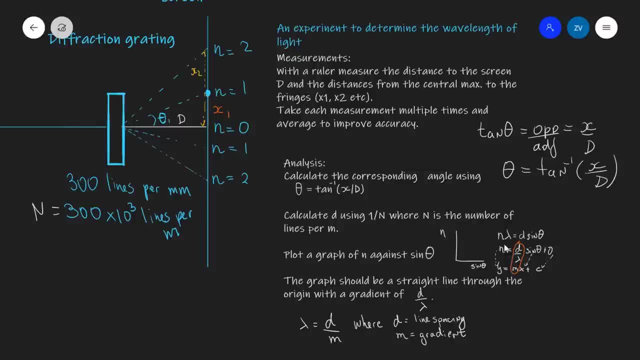 lambda. we just need to rearrange for whatever is on the y-axis And if we plot n on the y-axis sine of theta on the x-axis, our gradient is going to be d over lambda. The graph should be a straight line through the origin with a gradient of d over lambda. 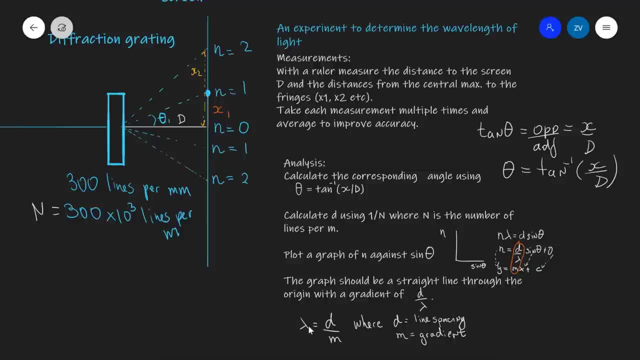 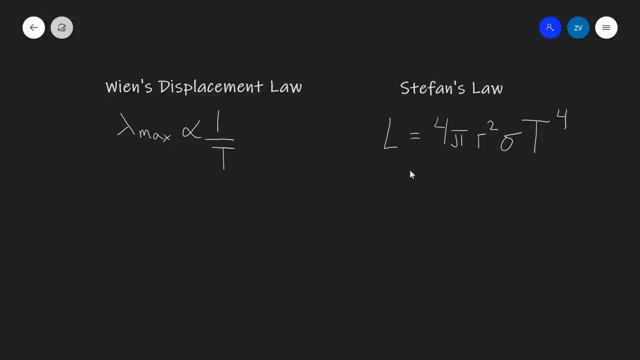 Just simply rearranging for lambda. we get that lambda. the wavelength will be equal to d, the line spacing divided by m, the gradient. We can use that to estimate its temperature and once we have its temperature we could even estimate its luminosity. 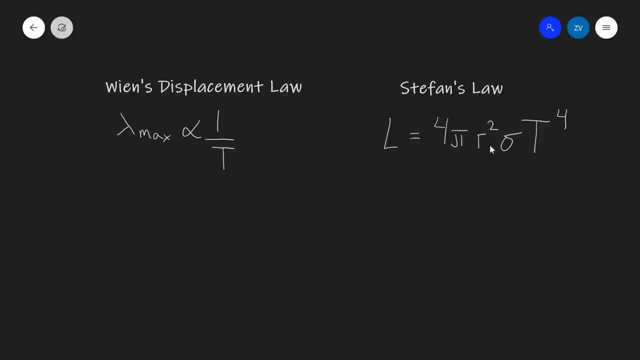 Or, if we have the luminosity, we could estimate the radius of a star. Let's start off by revising Wien's displacement law. This says that the predominant wavelength that's been emitted, lambda max, is inversely proportional to the temperature of the star. 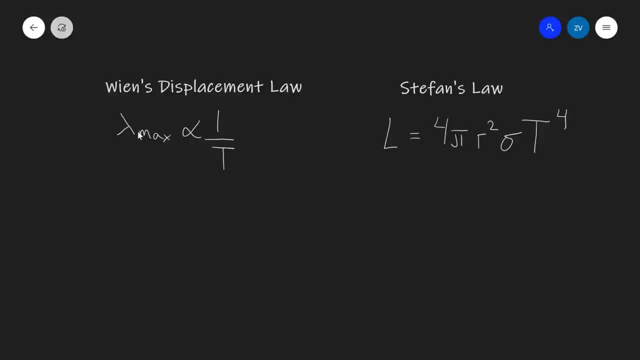 In practice, this means that stars with longer wavelengths, for instance red giants, are not going to be as hot, And stars with shorter wavelengths, for instance blue giants, are going to be quite hot. They're going to have a very high temperature. 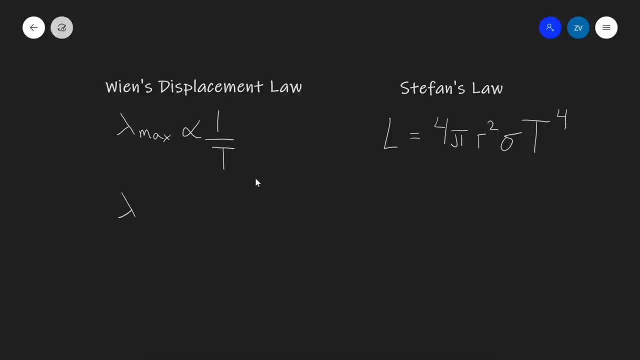 Mathematically, we could always write this statement as lambda max is equal to a constant. let's call that k divided by t. The value of this constant will either be given in the question or you need to be able to calculate it. 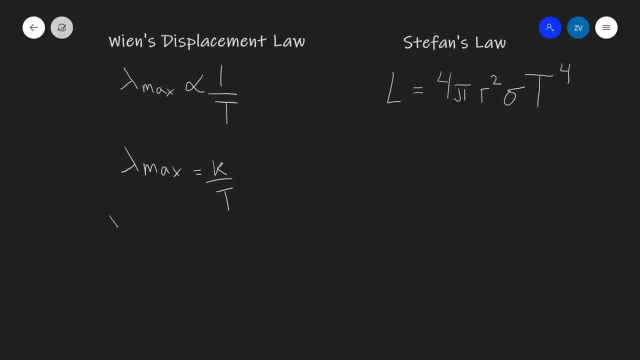 My favourite trick for this is simply just to say that lambda max times the temperature is equal to a constant where k is some constant. So we could always just write this down as: lambda max 1 times t1 is equal to lambda max 2 multiplied by t2.. 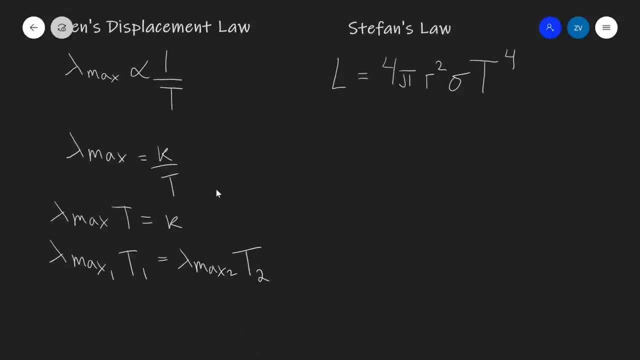 Now, moving on to Stefan's law. once we have the temperature, we could figure out really easily, let's say, the radius of the star. Just a couple of words about Stefan's law. first off, L over here, is the luminosity of the star. 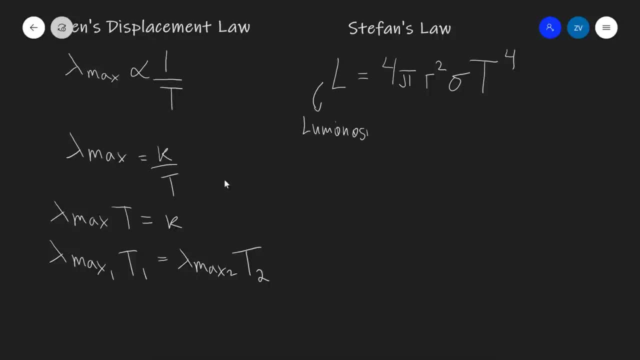 So luminosity of the star. Essentially, this is power, So this is measured in watts. It's the total power that's been radiated outwards from the star. 4 pi r squared, this is just the surface area of the sphere. 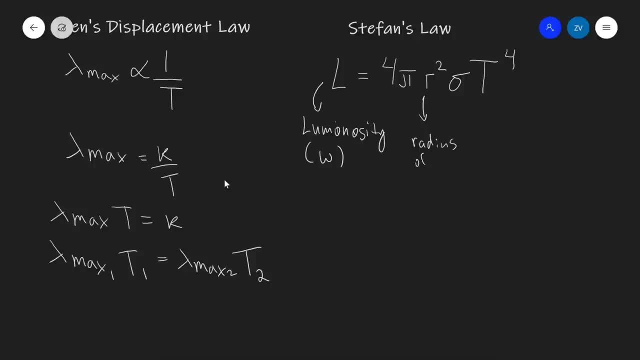 This over here is the radius of the star, Like so, And t is the surface temperature, Like so. Quite a common mistake would be to forget to raise this to a power of 4, or maybe square it. This is one of the few laws which is non-linear, and you can see that it's been raised to the power of 4.. 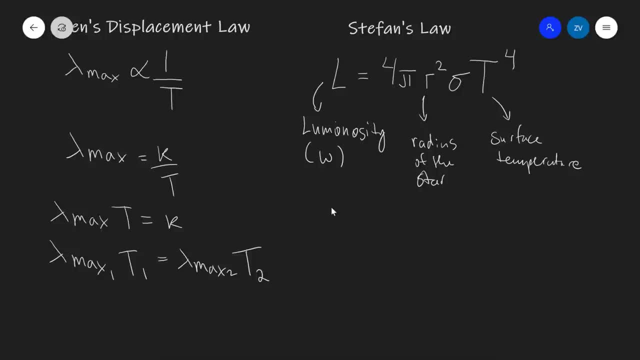 Okay, cool. Now let's quickly rearrange for r squared. for instance, if we wanted to figure out the radius of the radius of the star, r squared will be equal to the luminosity divided by 4 pi times Stefan Boltzmann's constant. 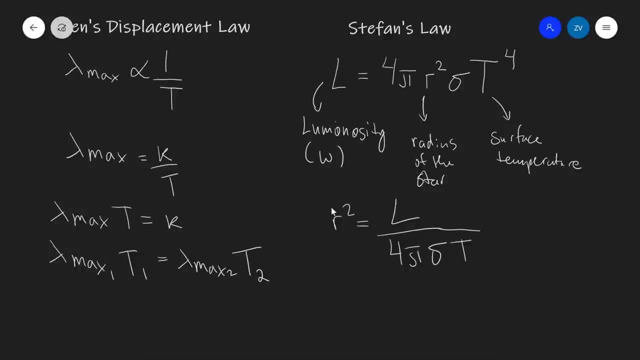 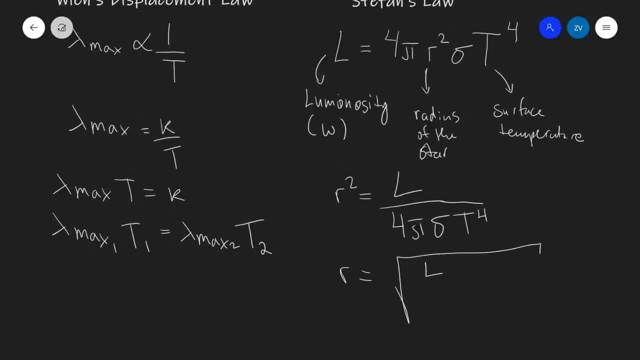 which is given in your formula booklet, multiplied by t to the power of 4, which means that the radius of the star will be given by the square root of L divided by 4, pi times Stefan's constant, times t to the power of 4.. 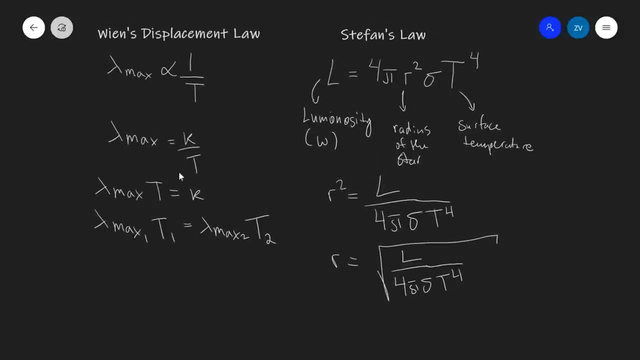 So quite a typical question would be to be given some data from which you would need to estimate the temperature of a star. Let's call that t2.. Normally you're given one set of data- lambda, max 1,, t1, then you need to figure out t2.. 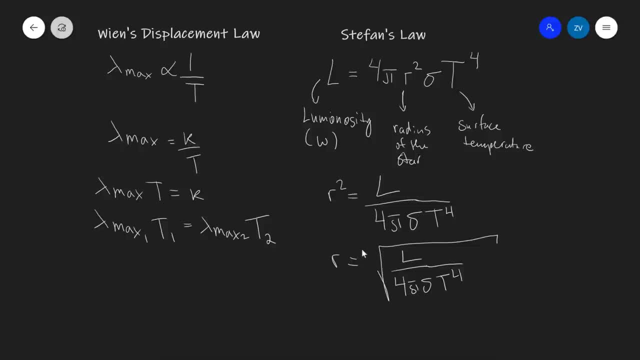 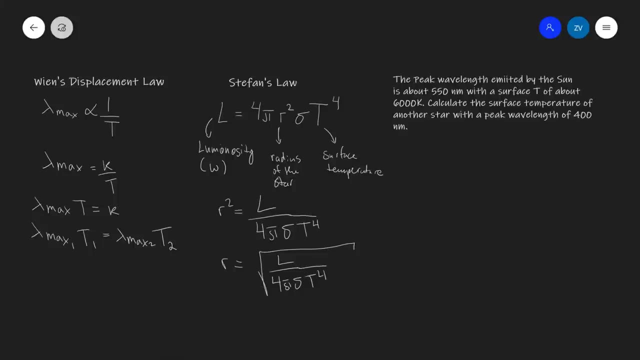 And then, once you have the temperature, you can use this equation to estimate the radius. Let's apply those two laws via an example. We have the fact that the peak wavelength emitted by the Sun is about 550 nanometers, with a surface temperature of about 6,000 Kelvin. 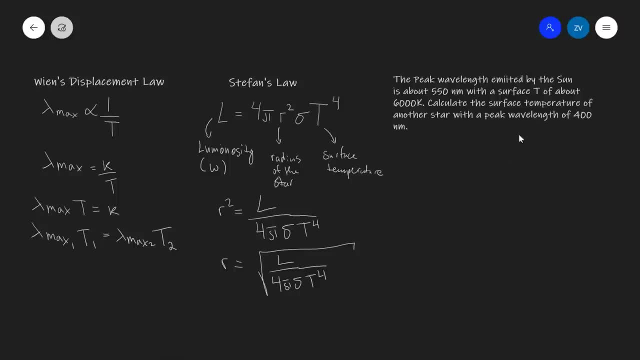 Calculate the surface temperature of another star with a peak wavelength of 400 nanometers. So in our formula booklet we know that lambda max is proportional to one over the temperature And as we've written down over here, we can always just say that lambda max 1 times t1 is equal to lambda max 2 multiplied by.